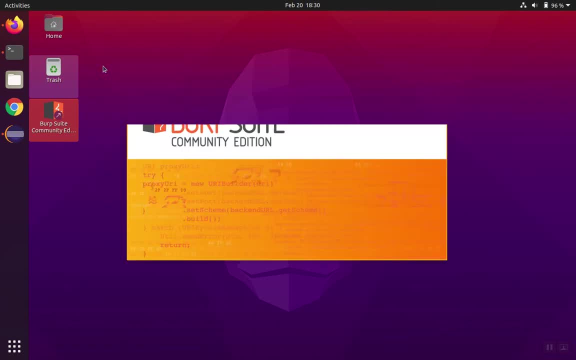 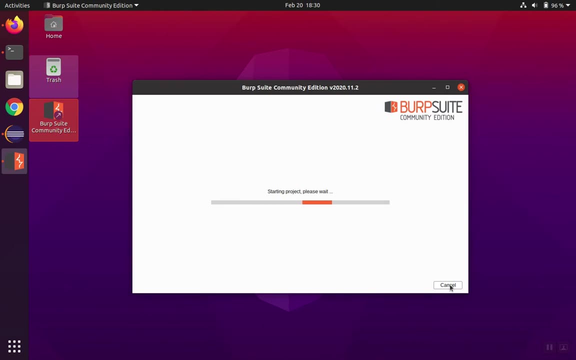 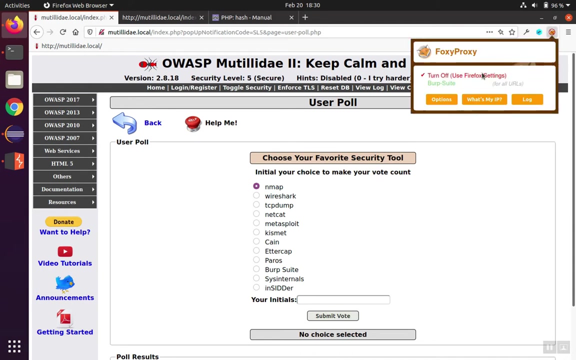 So we can watch the request and the token that we send can get sent and then we can watch the response that comes back. we have foxy proxy set up to proxy our requests over to burp suite that's listening on its default port with the browser using burp as a proxy. we'll submit the request. 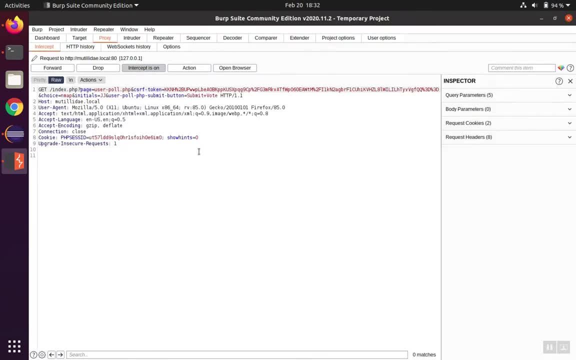 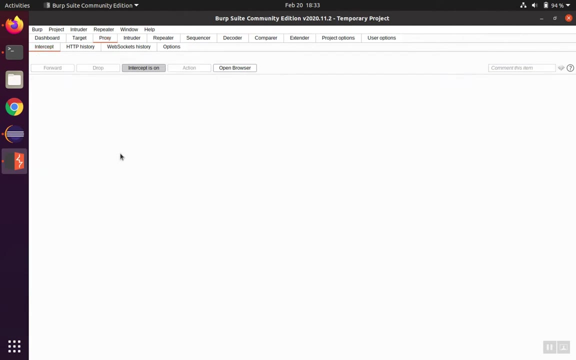 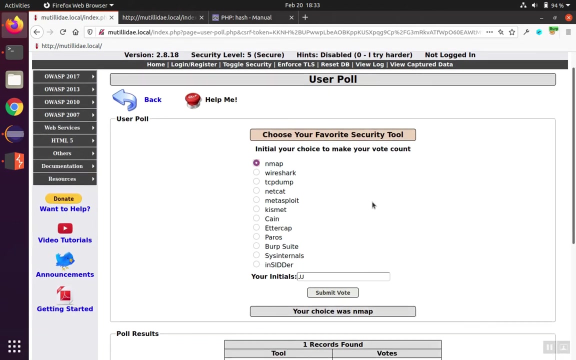 and we'll go over to burp suite to see the request. here's the token. now we're going to go ahead and let this go on to the server. the server will compare the token to the one that's in the session. verify that's a valid response and the page returns normally. this particular page. 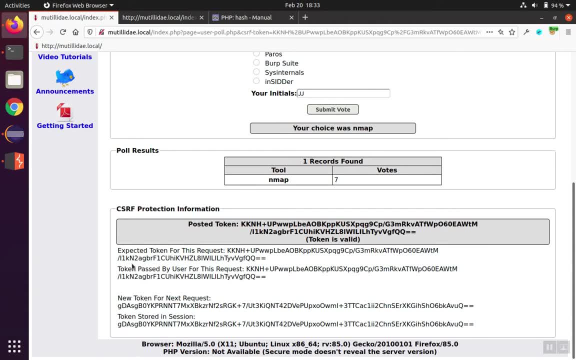 displays the tokens to make it easy to see what happened. so the server expected to get this particular token and that was the token that was passed by us over to the server. it's also put a brand new token onto the form. in case we submit the form again, it'll check. 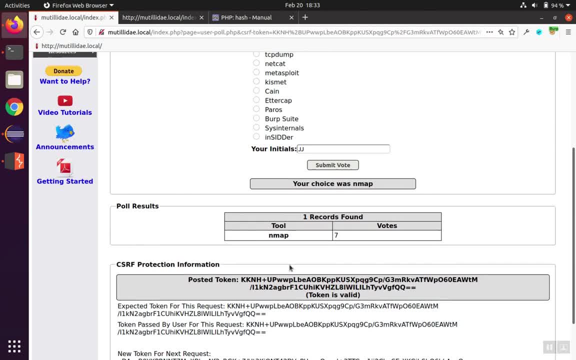 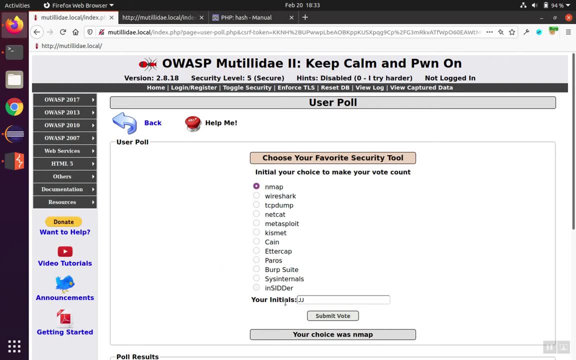 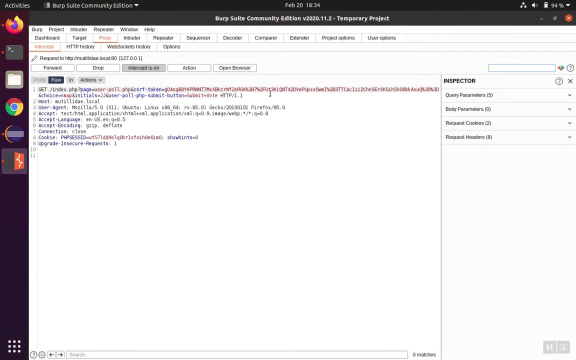 this against the token stored in the session, to make sure they match. so let's do this again, but this time we're going to change the value of the token and watch what happens. so we'll submit the form, but in burp suite we're going to go ahead and change the value of the token. 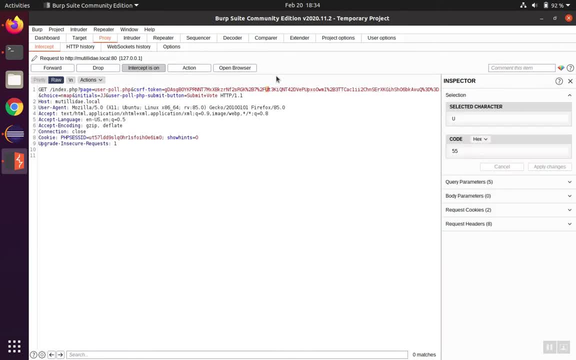 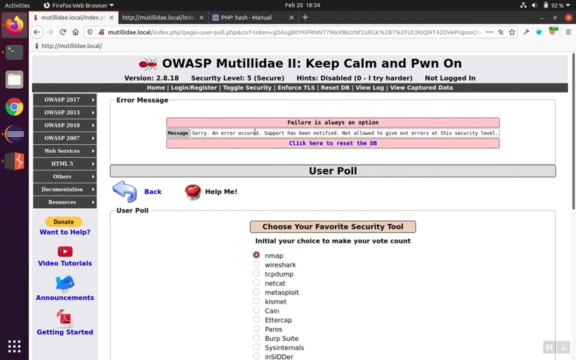 we don't need to make much of a change. we'll just change any particular character to something else, and then we'll just let the token go on its way. now we can see that the server was able to detect that the request was changed in some way. 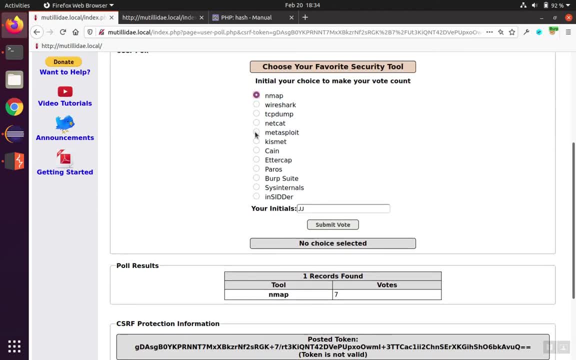 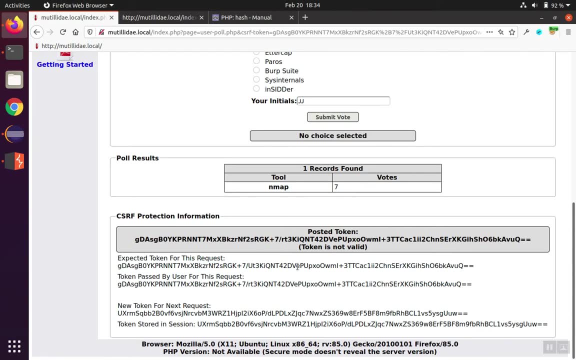 and went through and error, and this is because we changed one of the characters in the token. it expected to get token here, but instead it got the one that we had changed slightly because they didn't match. the server knew something was wrong and refused to fulfill the request. 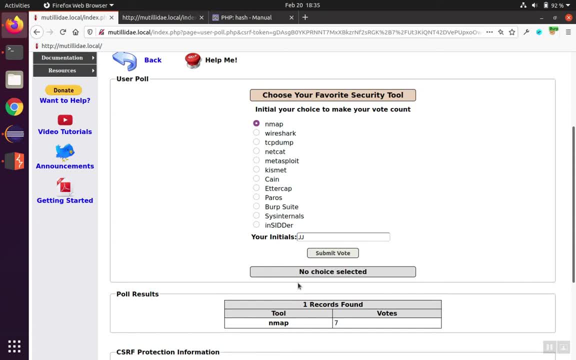 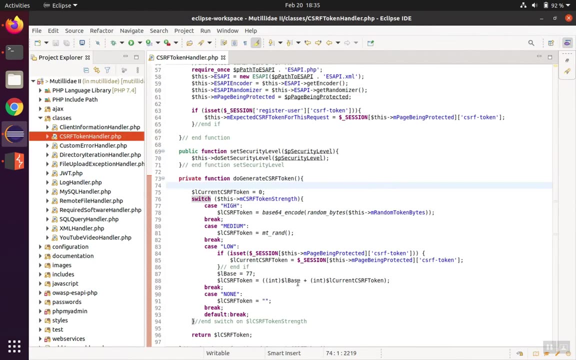 there's a few points about these tokens that we need to do when we're developing cross-site request. forgery defenses need to make sure that the tokens are cryptographically secure. random numbers- modern frameworks are capable of producing these types of tokens. just need to check which function to call in php. after version 7-3, we can call the random bytes function. 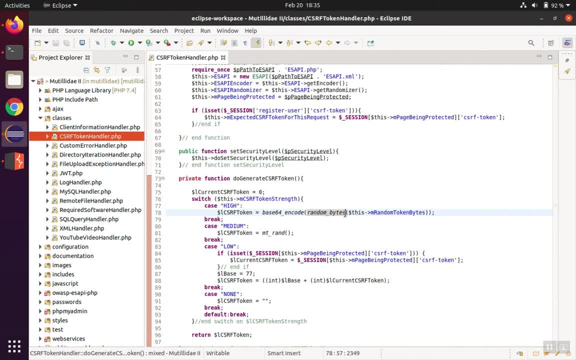 both java and aspnet have similar functionality, where they can generate cryptographically secure random numbers, but we also need to note that each of these languages also has a regular random number generator, and these standard random number generators don't necessarily generate truly random numbers. so mind the documentation and call the function that generates the cryptographically 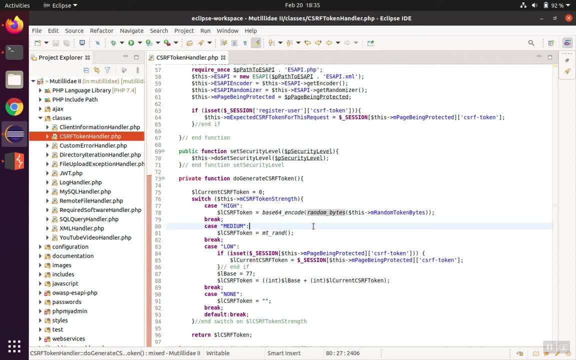 secure random tokens also make sure the token is long enough. several sources say that tokens that are 43 bytes in length should be strong enough to resist current attacks, and certainly if we just increase this up to the next power of two, which would be 64 bytes, that would seem to give us. 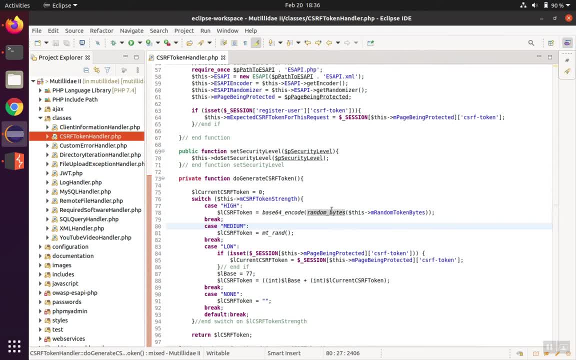 enough padding to be reasonably secure. most of these functions, like the ones in javanet and php, take in as an argument the number of bytes that you want to generate. usually, it's just a matter of passing in 64 in order to get back 64 bytes. 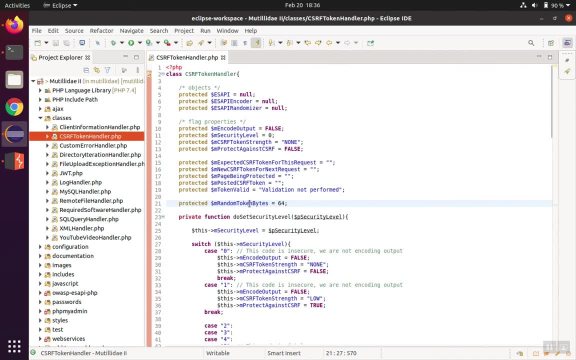 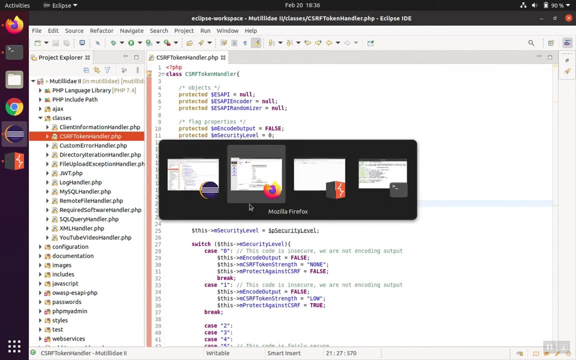 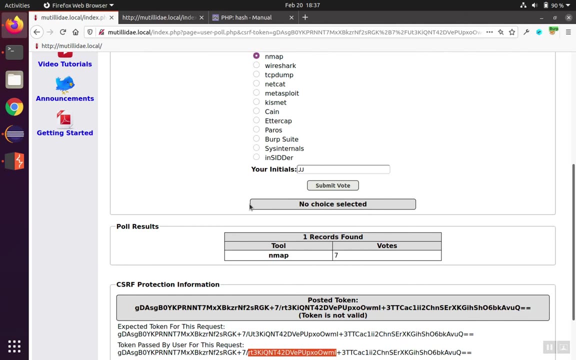 in this case, we've set the variable that controls the number of bytes to 64 to solve this particular problem. also, notice that our system is not reusing the tokens. we don't want to reuse the token more than once. the idea of the crossfire request forgery token is based on another concept called a one-time. 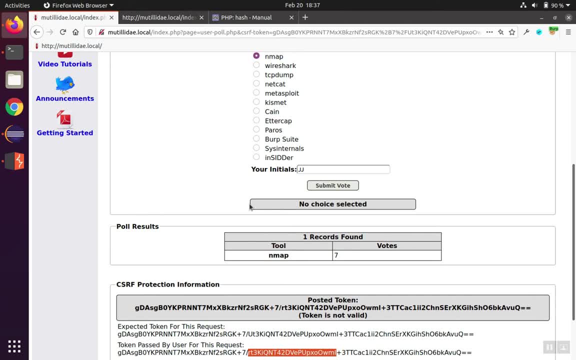 pass, and one of the key rules of a one-time pad is: do not reuse your key more than one time. this is because the secrecy of the system itself depends on the secrecy of the key, and so once the key's been used, it starts to become exposed and there's a greater chance that.